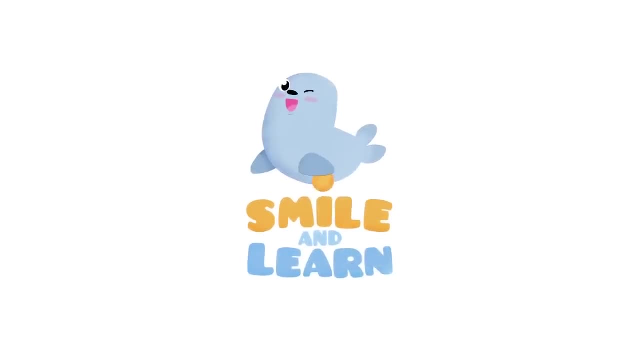 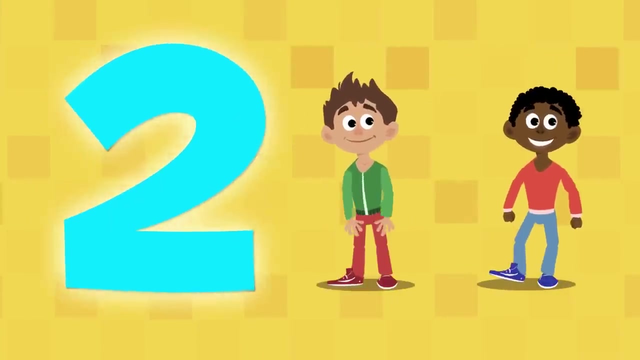 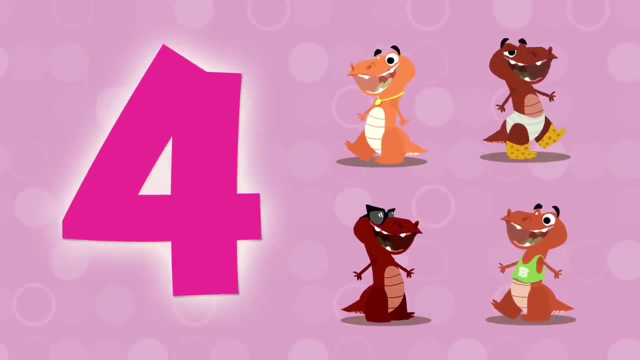 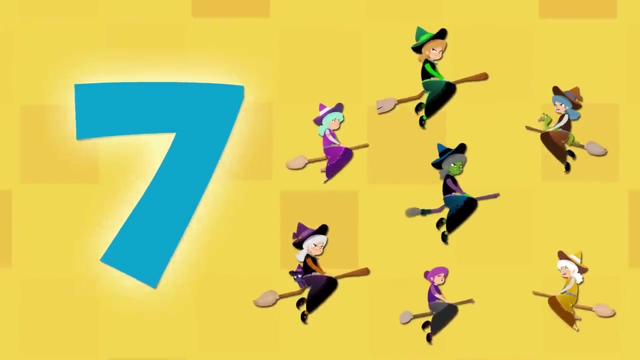 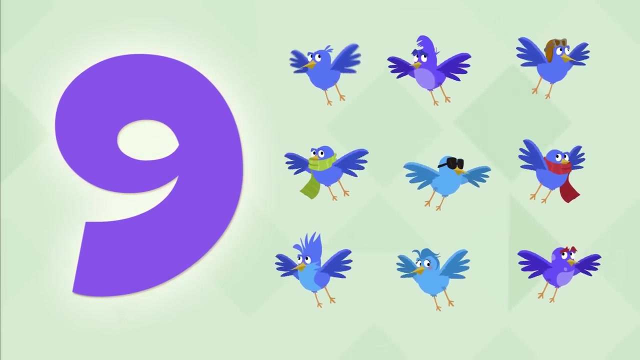 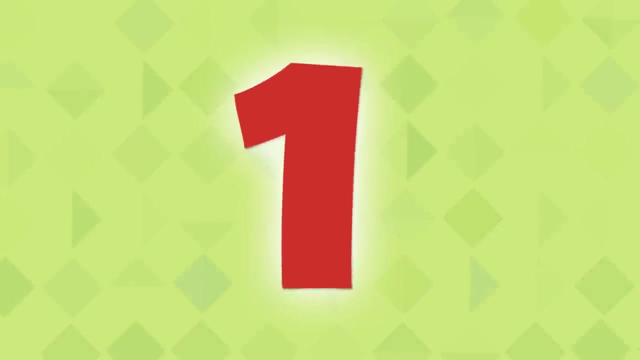 Hello, I'm the number monster. Do you want to learn to count? Pay attention: One, two, three, four, five, six, seven, eight, nine and ten. Let's try a little bit slower. This is number one. 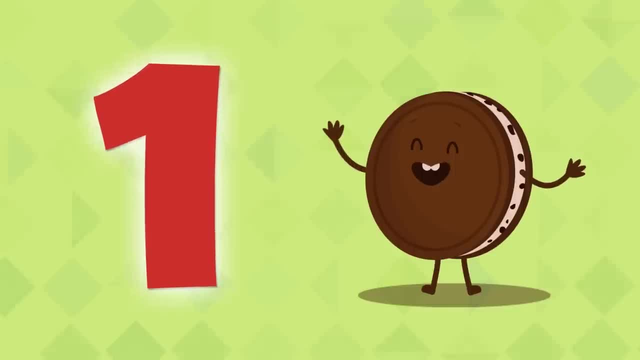 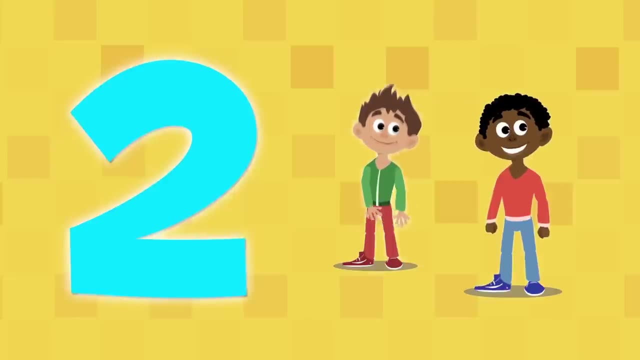 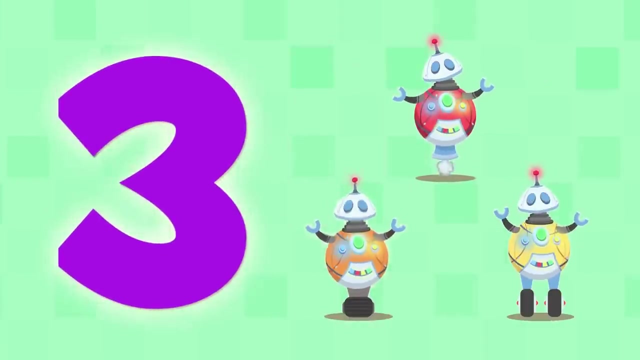 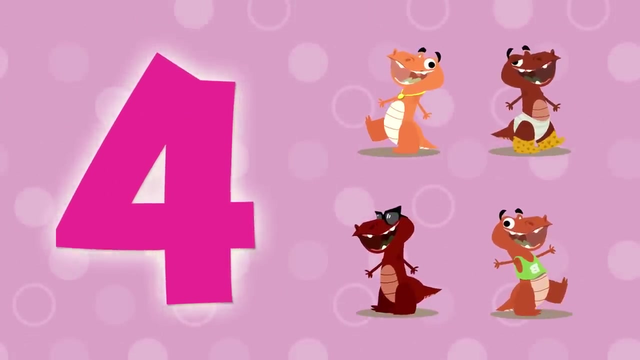 There is one cookie, Mmm, so delicious. This is number two. Here there are two kids, One and two. Here we have number three. There are three robots: One, two and three. This is number four. There are four dinosaurs: One, two, three and four. 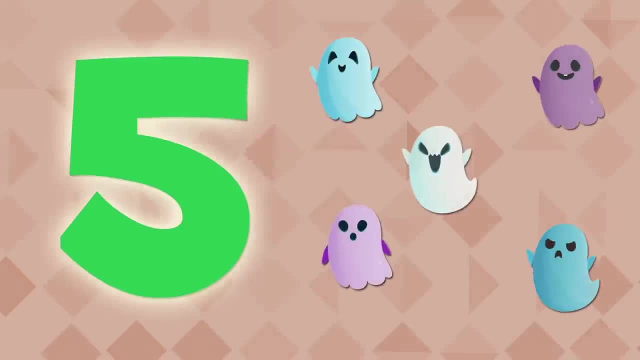 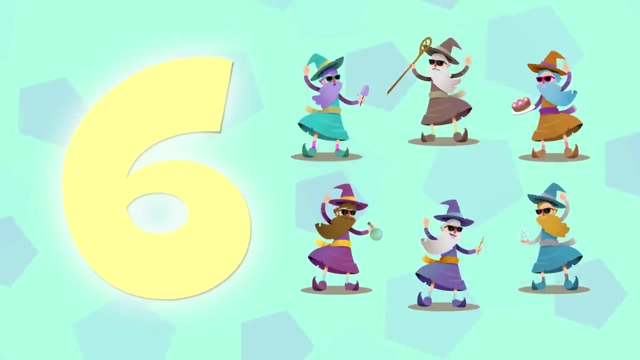 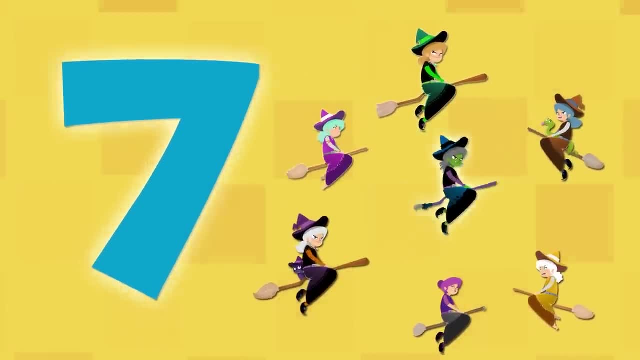 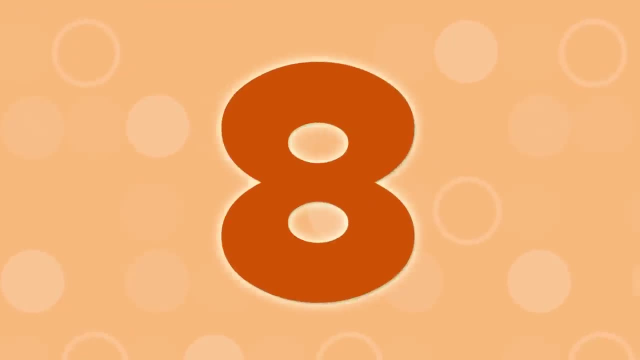 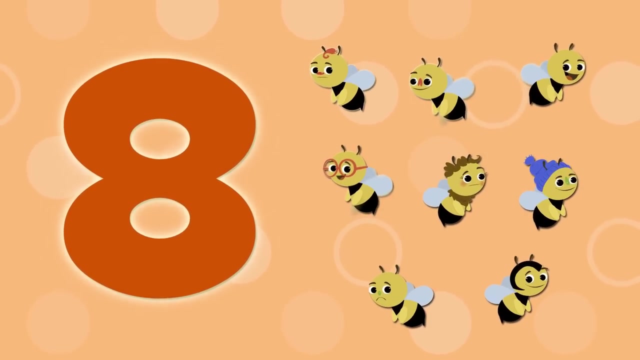 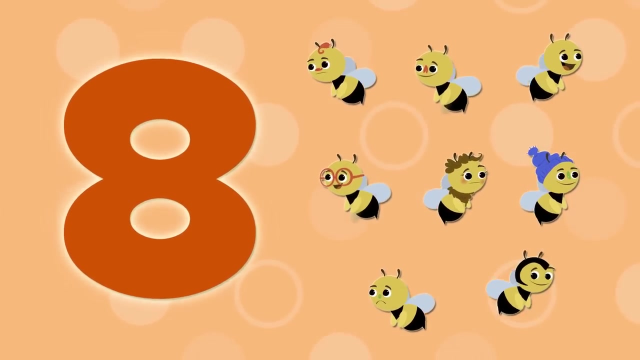 One, two, three, four, five, six and seven. Number eight is this one here. There are eight bees: One, two, three, four, five, six, seven and eight. This is number nine. There are nine birds. 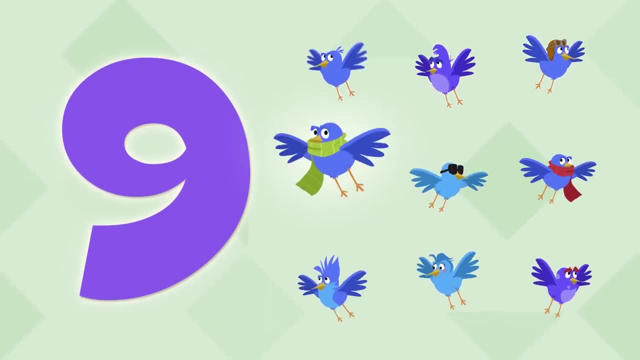 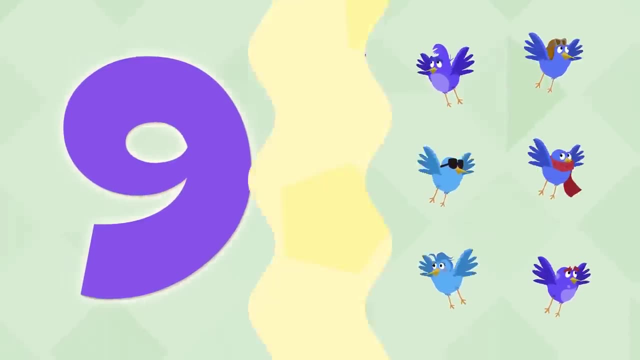 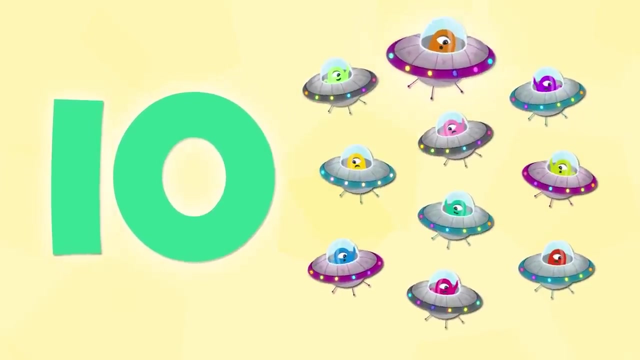 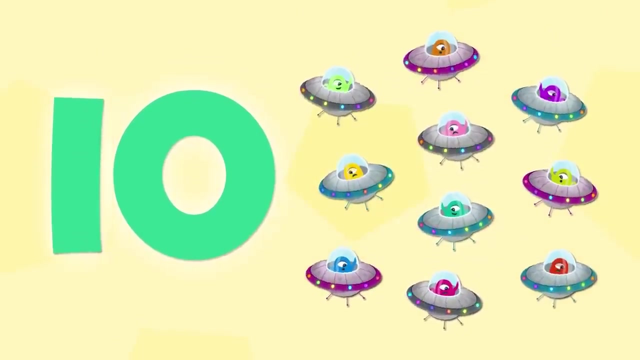 One, two, three, four, five, six, seven, eight and nine. The last one that we're going to learn is number ten. There are ten aliens: One, two, three, four, five, six, seven, eight, nine and ten. 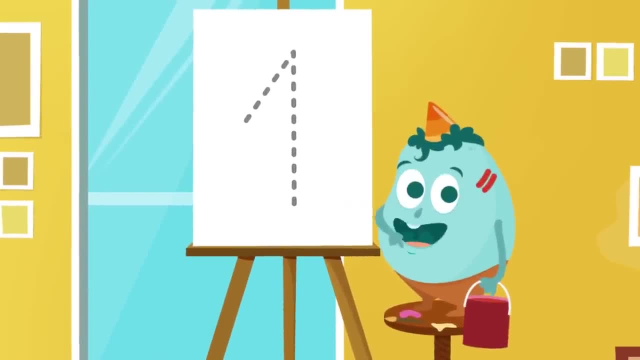 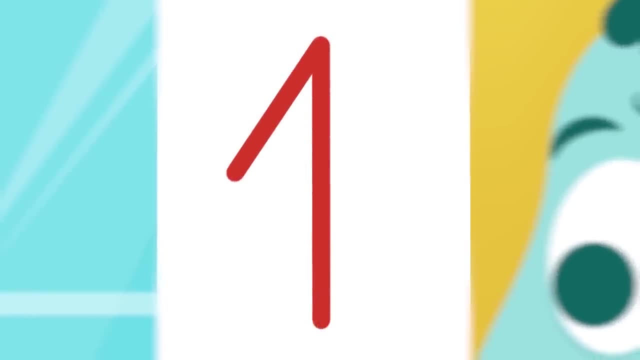 Hi, I'm the number monster And I will teach you how to write the numbers. Let's start here. We go up and now down here. What number is this Great? Let's see if you can figure out the next one. 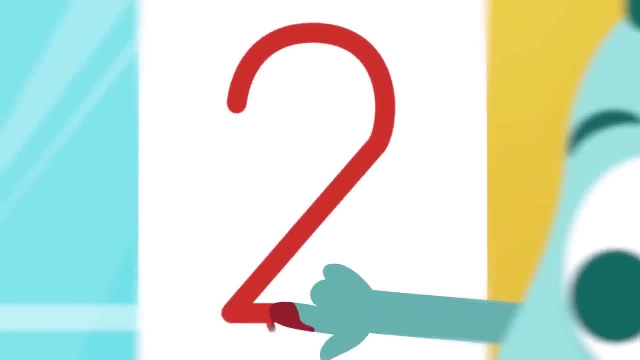 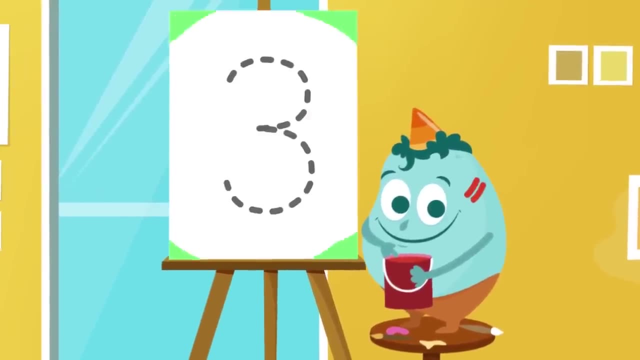 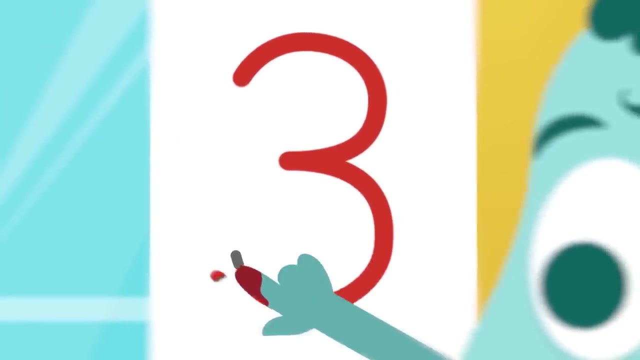 Let's make a curve like this and when we get to the bottom, we make a straight line to the right. What number is this? Perfect, We make this number like this: this small curve here and another similar curve here. can you figure out? 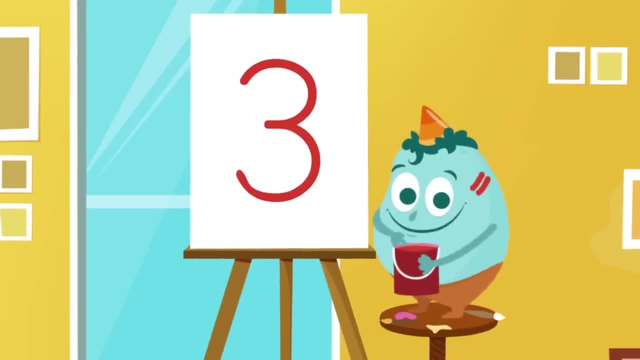 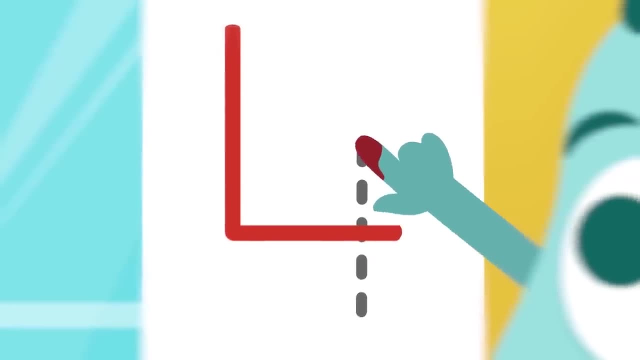 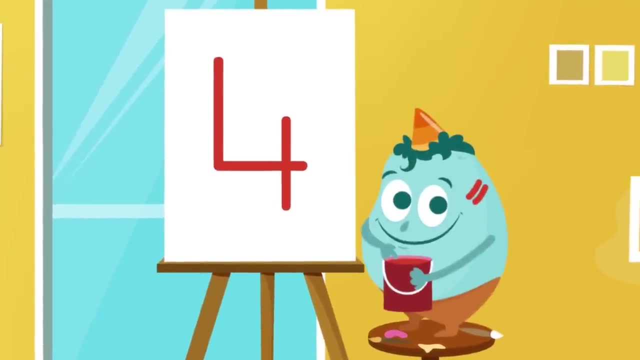 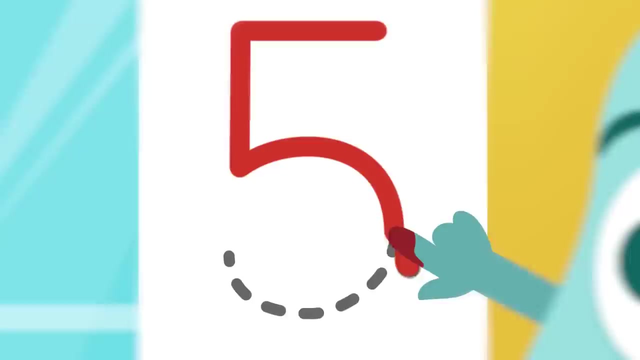 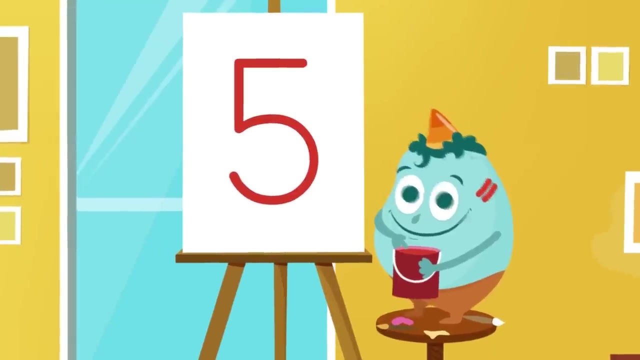 this number. let's do another one, a straight line here, then the next one here and then, to finish, one from here down. what number is this? let's do another one: a straight line towards the left, a straight line down, and now a curve like this, and this number, do you know what number is? very good, let's see if you. 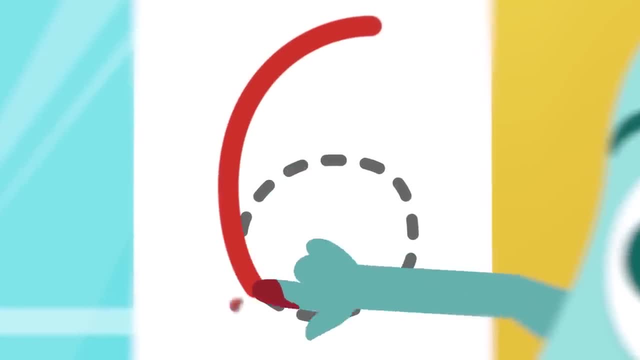 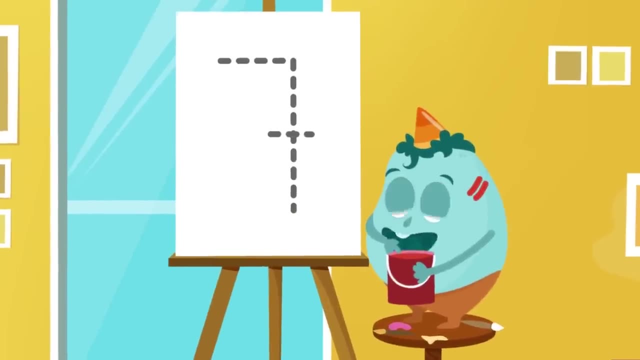 know this one. we start here, then go downward and we'll finish it by making a little circle. which one say, the next number has straight lines, born here, one that goes down here and last number straight lines? which one do you think is straight lines? and then across here a straight line and then a circle. 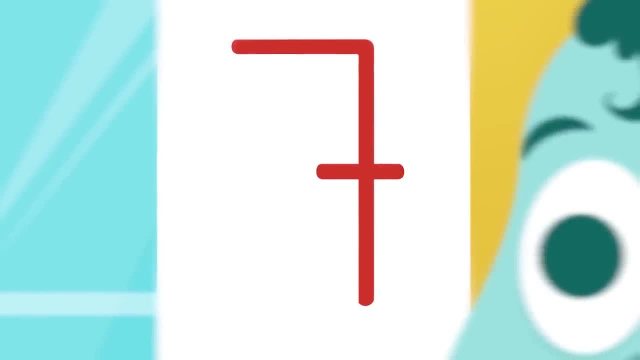 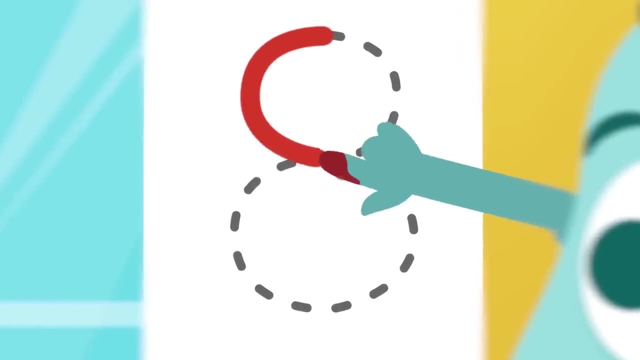 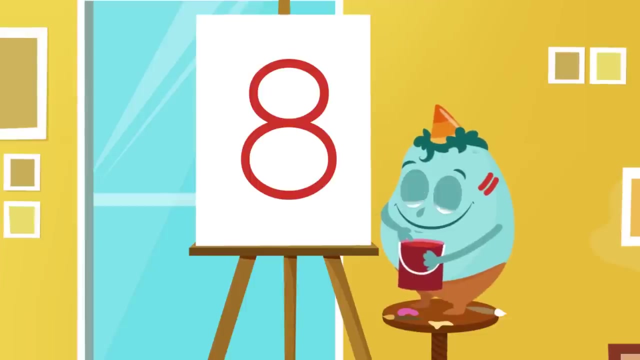 the small one that goes here. Now, do you know what this one is? Number 7!. Yes, Let's look at this one. Here. we make a small curve, then another one this way, and then we go up and do the same thing, And this number is Number 8!. That's it For the next number we